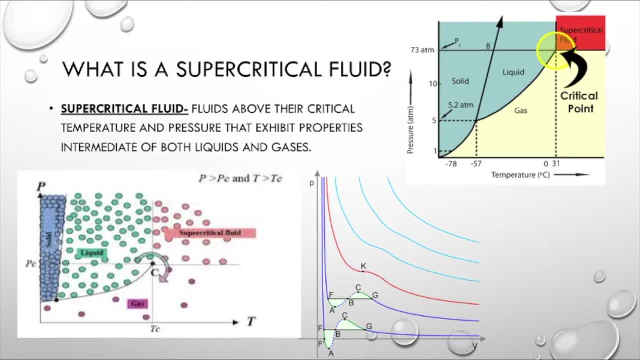 engineering. So let's get started. Okay, what is a supercritical fluid? A supercritical fluid is a substance that is subjected to a temperature and a pressure above its critical point. So these fluids exhibit properties intermediate of both liquids and gases. I provided here a few graphical 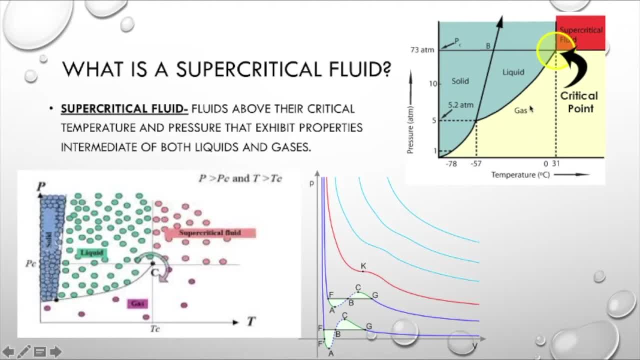 reminders of what supercritical fluids look like, which could be helpful. If you look over here on this first base diagram, you can see up here this: this red region represents the supercritical fluid region, whereas the critical point is right here. And if we look over here, I 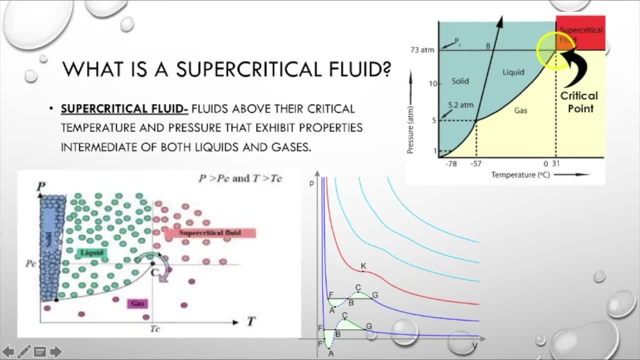 have this other phase diagram. We have it kind of just displays the this kind of you know this gradient of where certain regions of the supercritical fluid region represent more gaseous, you know properties. This region up here will be. 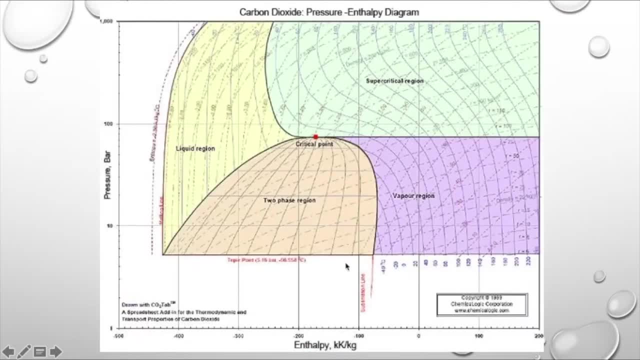 would be more resemblance of liquids. I've also provided this pressure versus enthalpy graph For another graphical reminder of where or how supercritical fluids, the supercritical region is shown up here in green where this critical point is, this point in red, right above the two-phase. 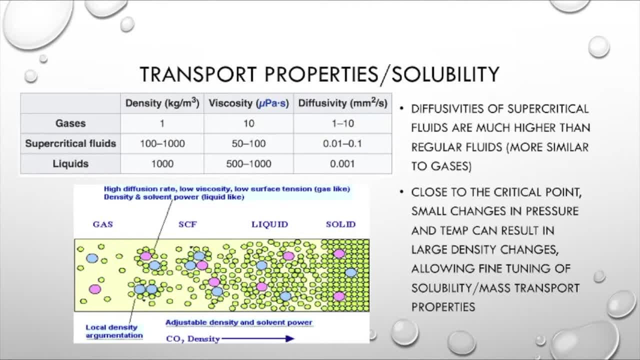 region, the vapor region and next to the liquid region. Okay, moving on to the transport properties and solubility advantages of supercritical fluids, Important point is the diffusivities of supercritical fluids are much higher than regular fluids. More resemblance to gases, actually, You can see that in this. 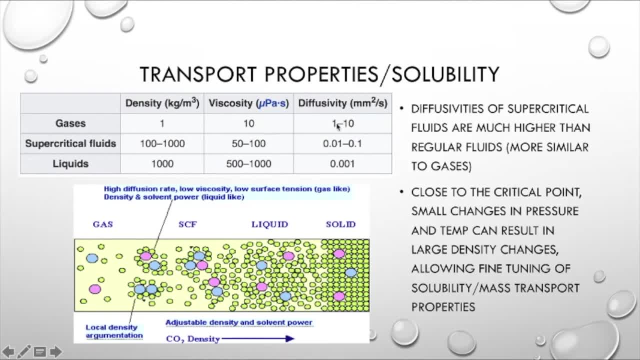 this graph over here. I've shown- or this is for this table over here- that the diffusivity constants of gases for critical fluids liquids, you know, comparing them, also the densities and the viscosities. This increase in diffusivity is a huge advantage over the liquids as it improves solubility. 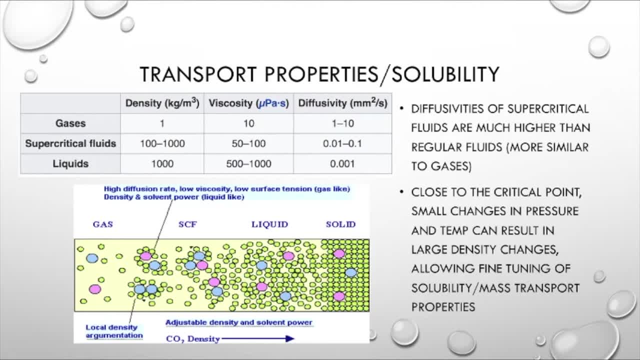 properties of the fluid by a substantial degree. Solubility is usually an important property to consider in chemical to chemical engineers, especially in the case, you know, if we're talking about mass transport effectiveness, In order to achieve the selectivity and yield structures that we typically want. 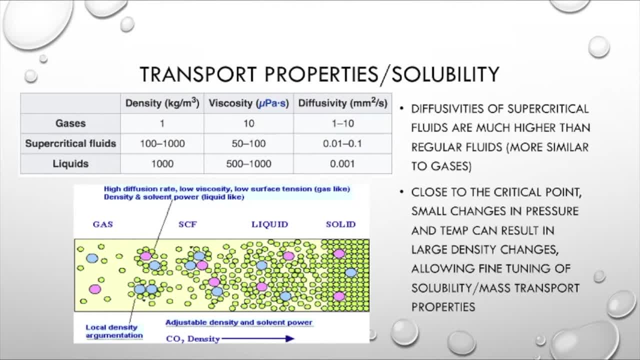 from a separation or need for a process. we want to be able to fine-tune the solubility of the working fluid that's in the process. So you know, being able to have this advantage or this, this diffusivity increase, is a huge. 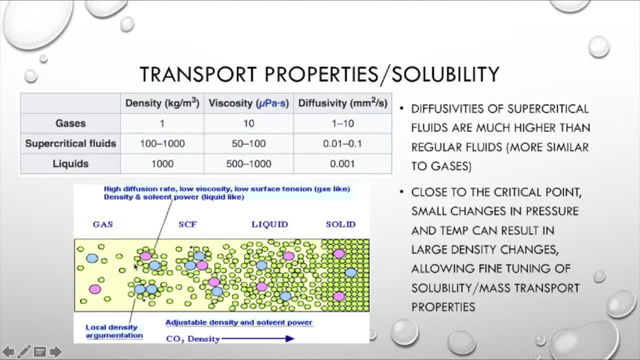 advantage. The diagram down here you know kind of shows this molecular solubility difference, you know as a gradient from solid to gas. You know we take note into how this you know the supercritical fluid is between liquid and gas and adjustable density and solvent power, Another important 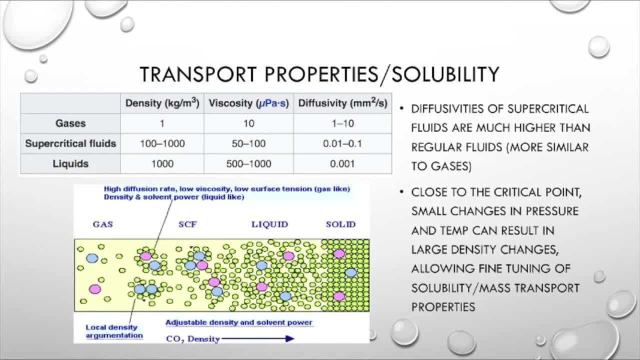 point to note is when close to the critical point, small changes in pressure and temperature can result in large density changes, which is important because it allows us to to fine-tune these solubility and mass transport properties more more exacting or more precisely, So shown here are. 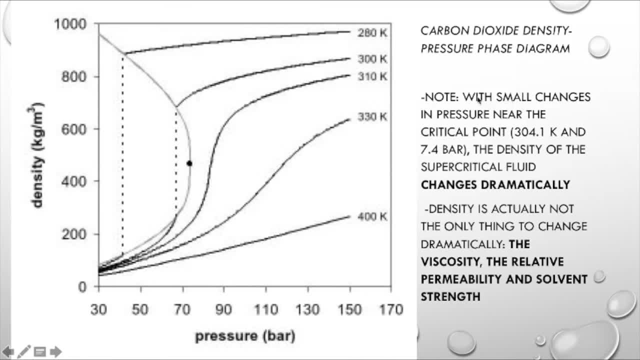 we have the carbon dioxide density pressure phase diagram. This is also just repeating this point, you know, showing that whenever we're close to this critical point, right here, the density is, you know, changing very rapidly, especially on this 310 isotherm. It's important to note that the 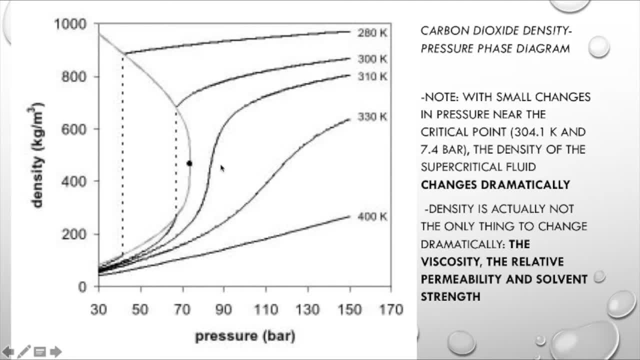 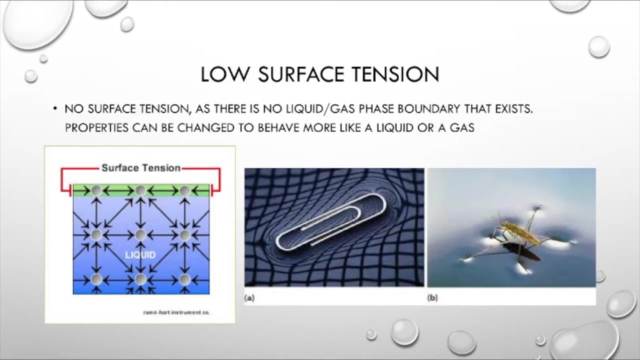 density is not the only thing that changes dramatically close to the critical point. Also, the viscosity, the relative permeability and the solvent strength also change to a notable degree. Okay, Another important advantage to consider is the low surface tension that is found within. 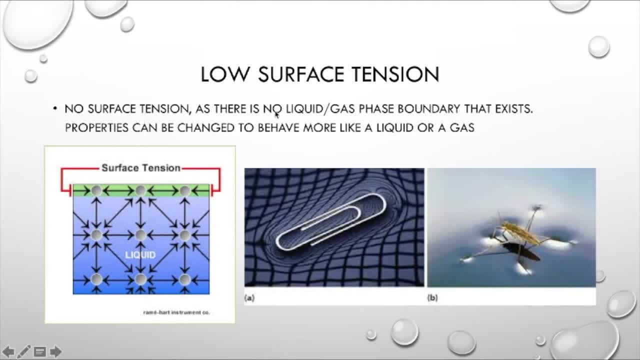 supercritical fluids Almost no surface tension as there is no liquid gas phase boundary that exists. This is helpful in making the fine-tuning of the solubility easier and allows for better pore penetration whenever we have some kind of any kind of solid matrix or mass transport. 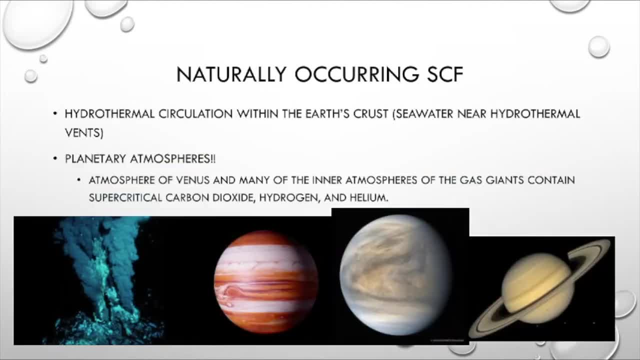 matrix that we need to to work with Some naturally occurring supercritical fluids which I thought were kind of cool. they exist in hydrothermal vents or in the seawater around hydrothermal vents and within the inner atmospheres of some of the planets in our solar systems most. 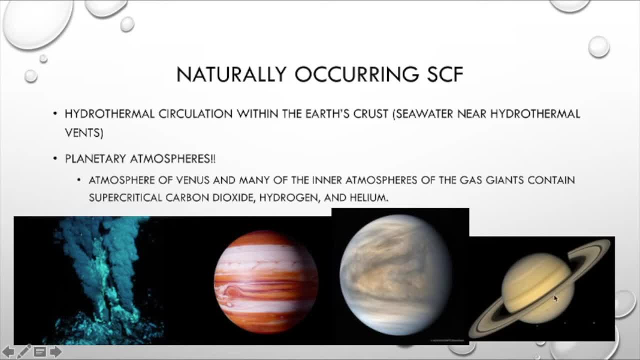 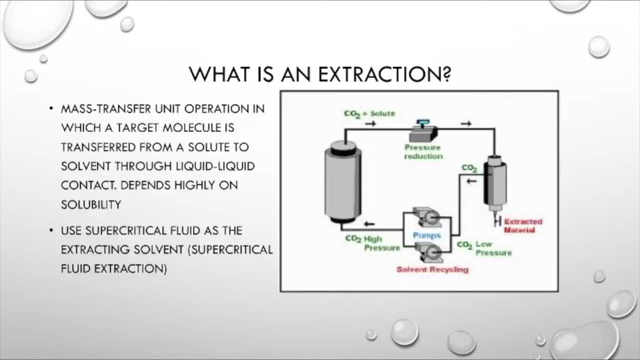 notably Venus, Jupiter and Saturn. Temperatures and pressures of these regions are just right for supercritical fluids to form, and they exist in that region. Now let's consider what is an extraction and how is this, you know, connected. Now let's consider what is an extraction and how is this, you know, connected. 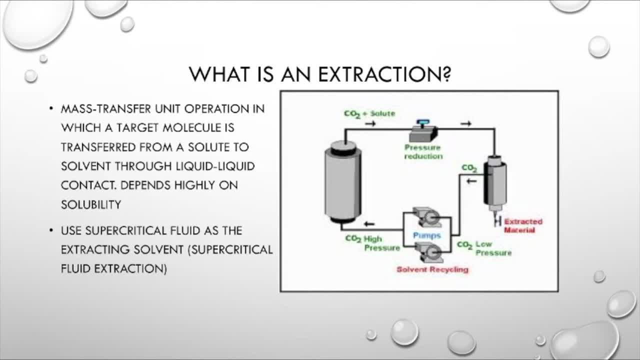 Now let's consider what is an extraction and how is this, you know, connected? A liquid-liquid extraction involves the mass transfer of a target molecule between a solute and a solvent. The effectiveness of this process depends highly on solubility limits and the properties of the working fluids. 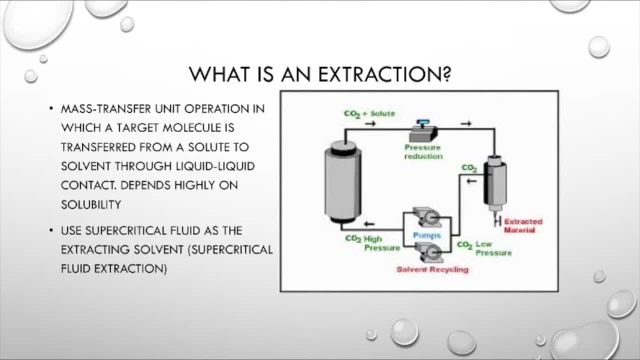 involved. Generally, it's best to maximize solubility of the solvent if one wants to achieve, you know, a maximum mass transport between the fluids. Regular fluids usually don't always cut it. They have undesirable solubility properties needed, you know, or they can't really achieve a high. 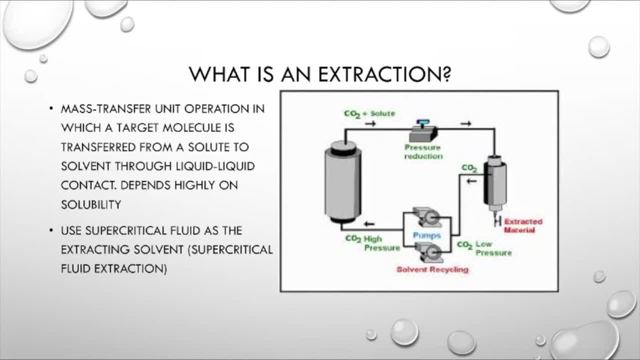 yield of mass transfer due to the constrictive diffusivity limits. That's where the supercritical fluids are advantageous. If a supercritical fluid is used as the extracting solvent, a supercritical fluid extraction can be performed, which you know. as discussed previously, these supercritical 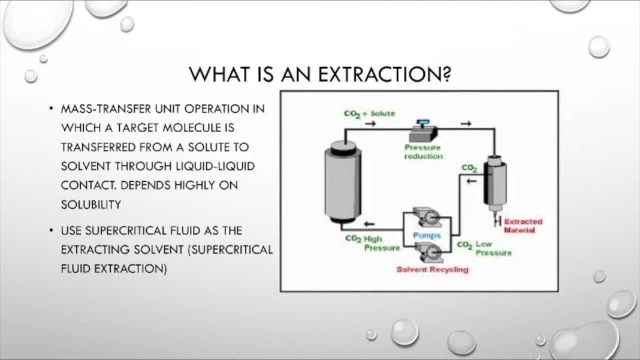 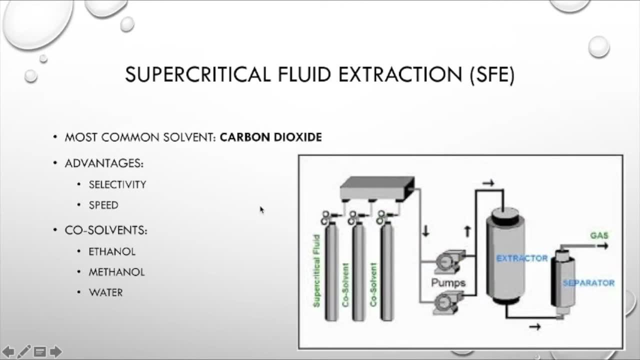 fluids. they have much higher yields and selectivities due to the distinct property differences from regular fluids or regular liquids. Okay, just going to briefly mention the basics of supercritical fluid extractions and their advantages over regular extractions- The most common solvent used in practice in industry is supercritical. 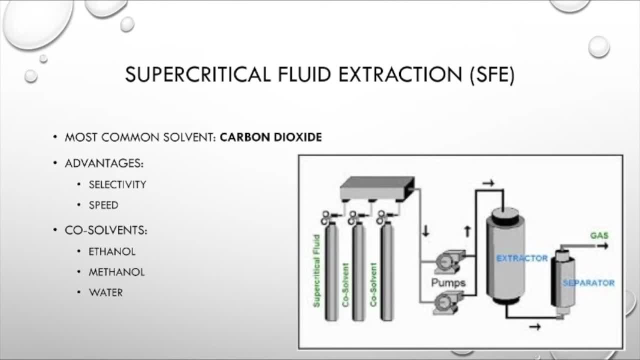 CO2.. Why CO2?? Well, a few reasons. It has low critical pressure and temperature, it is relatively nontoxic, it is non discutable and it's easily available to experimenters in pure form, such as in dry ice and pressurized CO2. 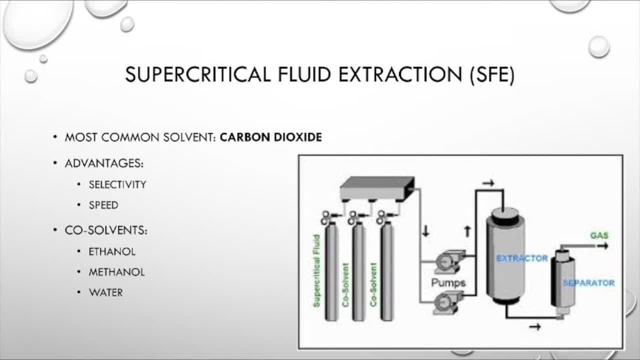 tanks. The overall advantages of SDFEs are the selectivity and speed improvements over regular extractions, which is due against the differences in diffusivity properties. Typical co-solvents used in industry are ethanol, methanol and water, which are used to enhance the solubility power of CO2,. 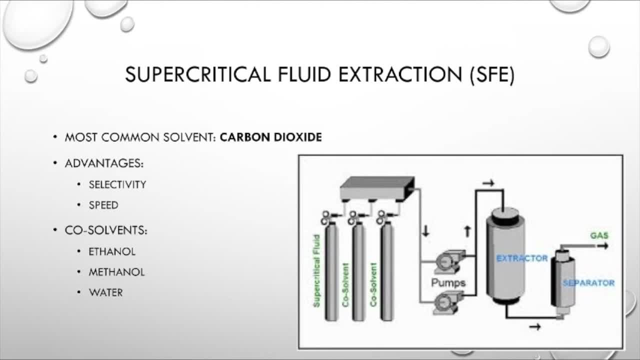 making it possible to extract much more polar molecules from a solvent or from a molecule of interest. The diagram here shows a typical process of an SFE. As it can be seen, the supercritical fluid is mixed along with the co-solvents or pumped in to the extractor tank and then, after 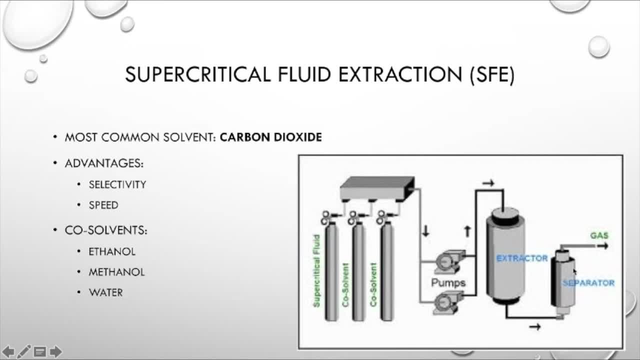 it is sent to a separator where further purification is performed. Sometimes a heat exchanger is included along here or before the extractor just to ensure that the supercritical conditions are met within the fluid before the extraction occurs, As we'll see in the next few.